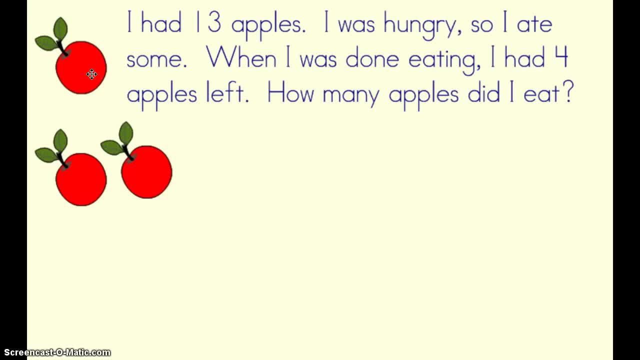 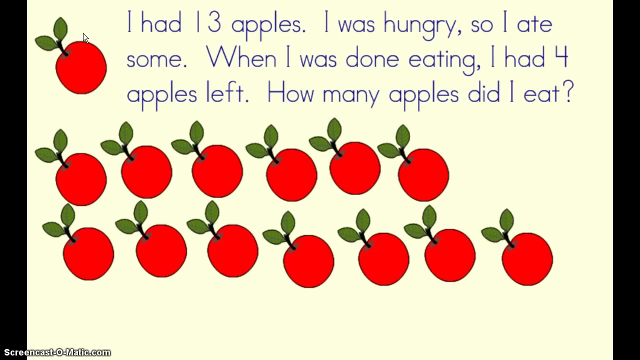 One, Two, Three, Four, Five, Six, Seven, Eight, Nine, Ten, Eleven, Twelve, Thirteen. I had 13 apples. I was hungry, so I ate some. In this problem, some is a number, but we don't know how many it is, so we need to keep reading. 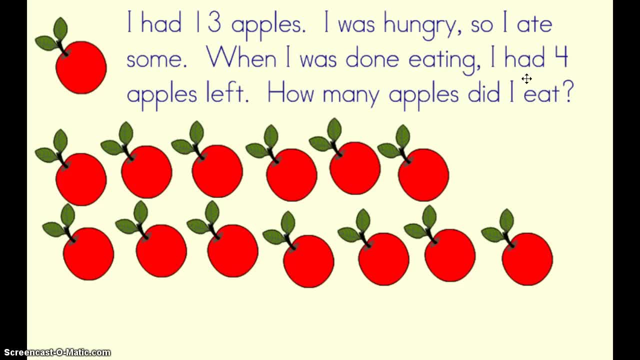 When I was done eating, I had 4 apples left. That means I want to eat some apples, but when I'm finished there still need to be 4 left that have not been eaten. To do this tonight, I'm going to cross out some of my apples at the end. 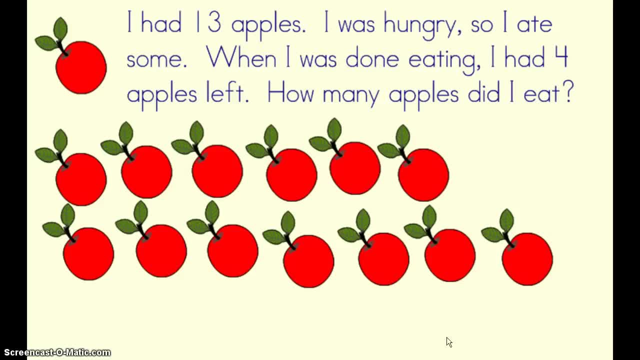 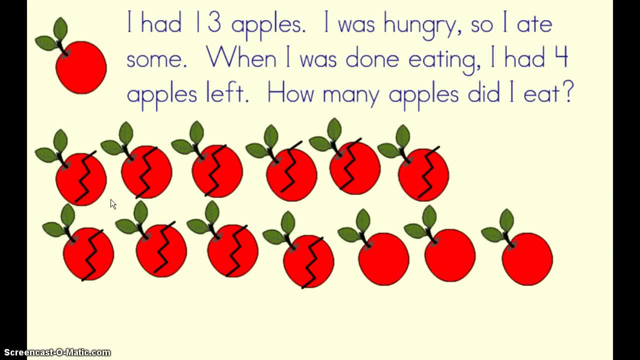 I was hungry, so I ate some. Yes, I did. When I was done eating, I had 4 apples left. When I was done eating, I had 4 apples left. When I was done eating, I had 4 apples left. 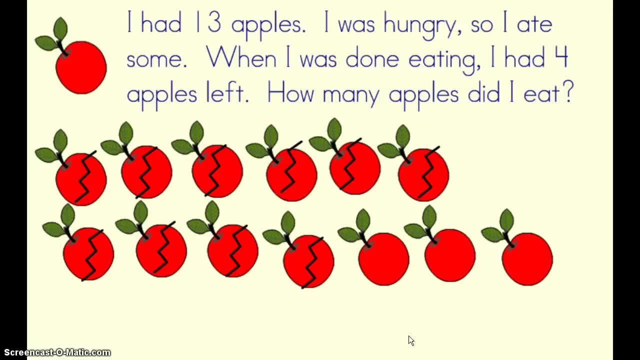 Do you see a mistake that I made? Do you see a mistake that I made? That's right, I only have 1 apple left. 1, 2, 3 apples left. 1, 2, 3 apples left. 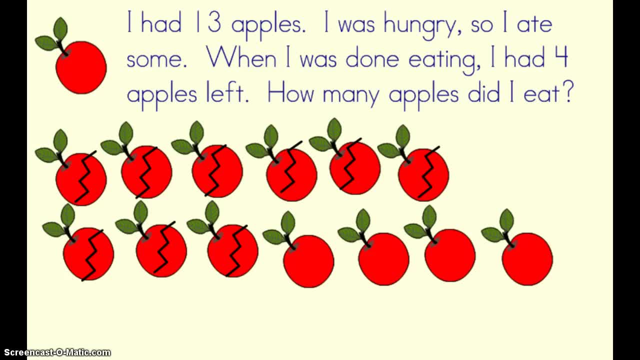 I need to get rid of 1 of my crunches. I need to get rid of 1 of my crunches Now. I have 4 apples left. Now, I have 4 apples left, And that's what the story problem tells me. 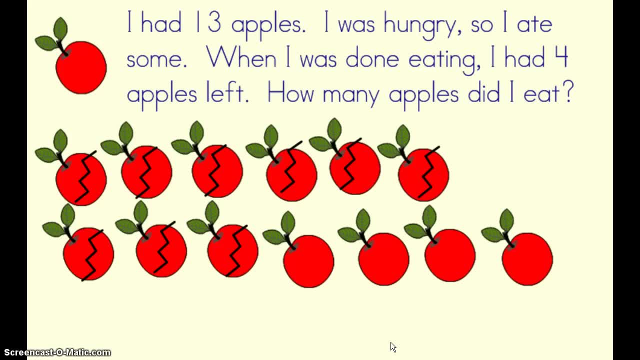 Now I need to make sure that I answer the question. Now I need to make sure that I answer the question, Because I have not done that yet. My question asks: How many apples did I eat? Let's count how many apples I ate. 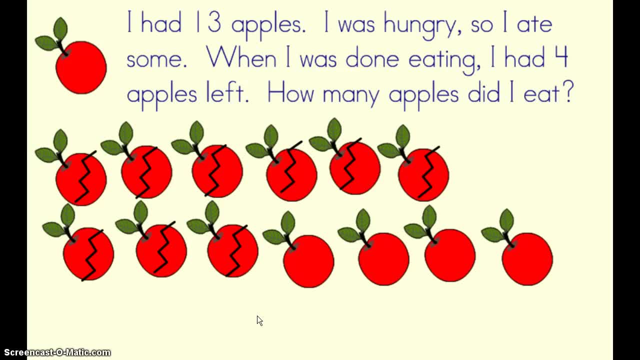 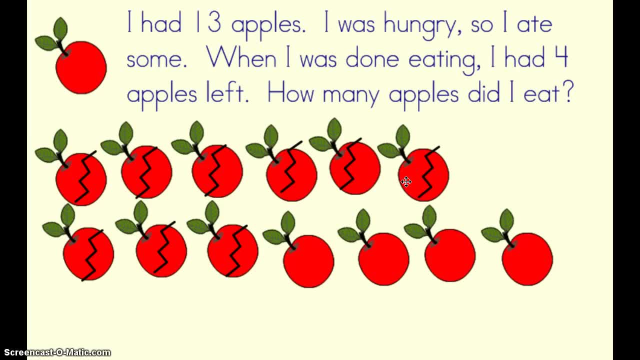 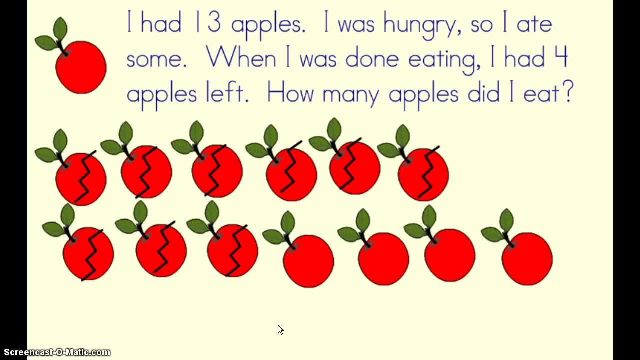 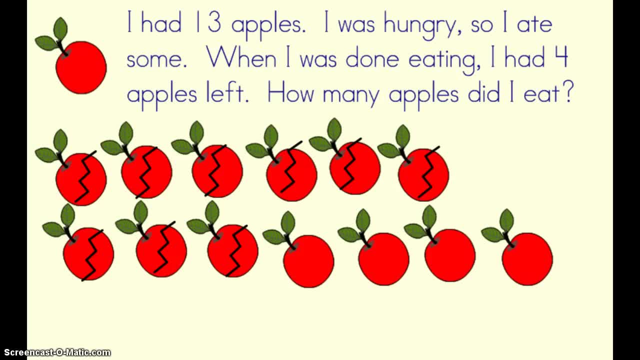 I'm going to write a sentence to answer this question. I'm going to write a sentence to answer this question. I eight nine apples period. it's important when we're reading a subtraction problem, to make sure that we understand what we're reading and that. 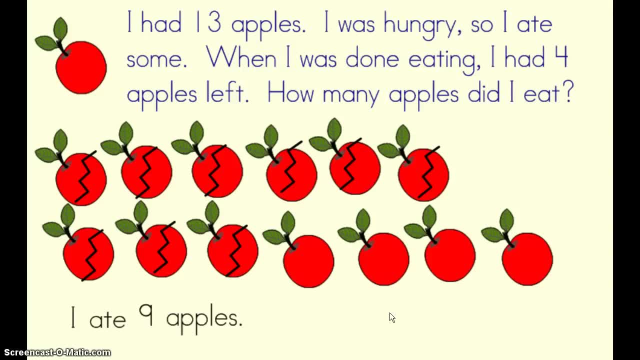 we answer the question that is being asked. I'm going to double check my work just to make sure I had 13 apples: 1, 2, 3, 4, 5, 6, 7, 8, 9, 10, 11, 12, 13. I was hungry, so I. 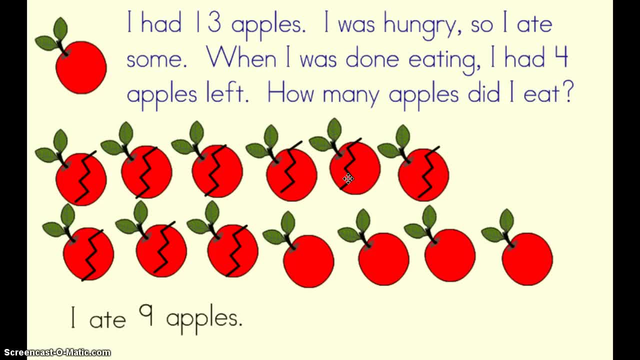 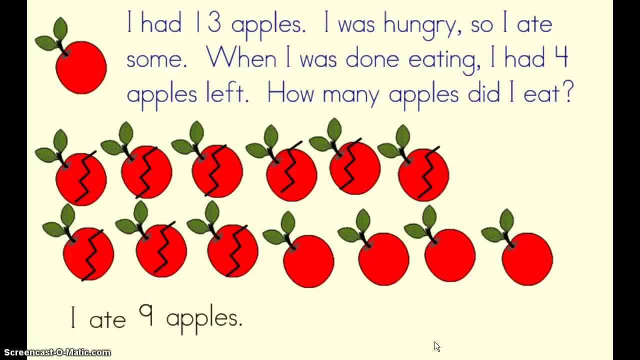 about a different way you could solve this problem. Tomorrow in class we're going to talk about other ways we can do this. We might use a picture. We might write a subtraction sentence. We could also write an unknown number addition sentence. Tomorrow in class you will talk with 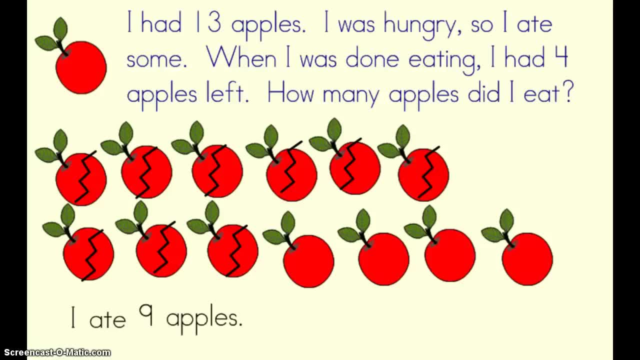 your teacher about some of these ways. See you then, you.